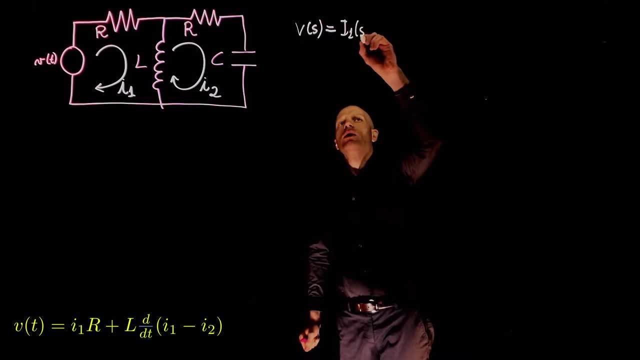 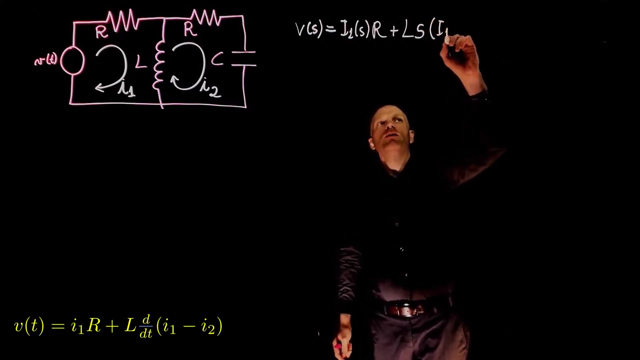 I of T becomes I1 of S times R plus the voltage drop across the inductor, that is the inductance times, the derivative of the current. The current in this case is I1 of S minus I2 of S And you notice S here. 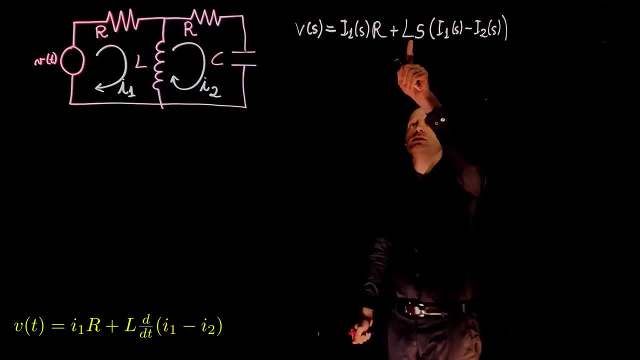 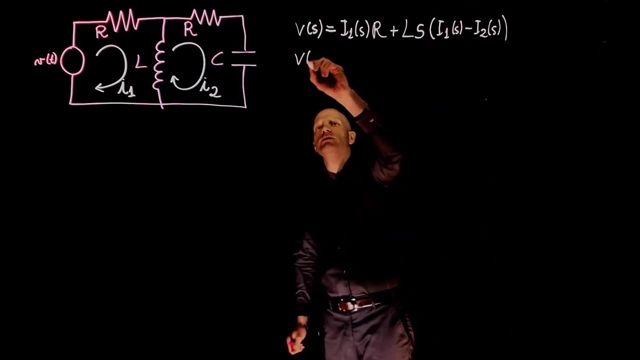 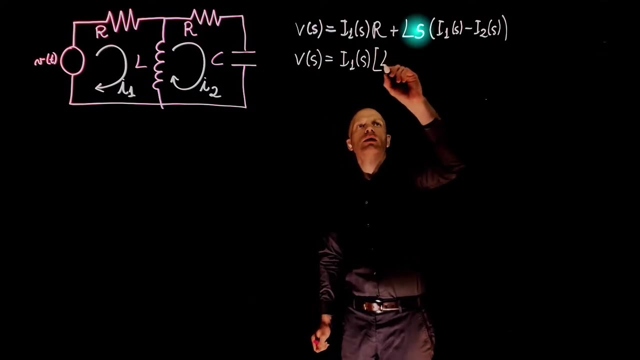 S represents the derivative in the frequency domain, So the inductance times the derivative of the net cart. We can now factor I1 of S in this equation and rewrite it as V of S equals to I1 of S times Ls plus R. 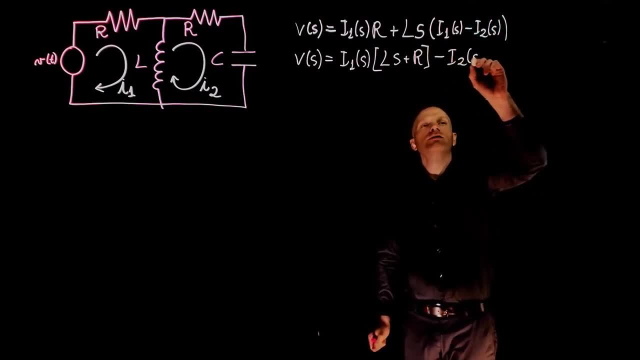 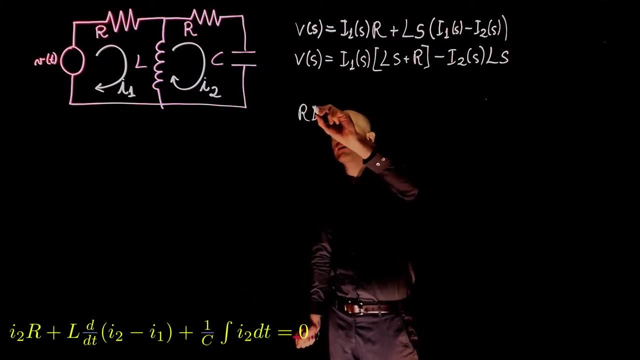 minus I2 of S times Ls. For the second loop, let's start with the resistor. The voltage across the resistor is R times I2 of S. The voltage drop across the capacitor is 1 over C times the integral of I2.. The integral in the frequency domain is 1 over S. 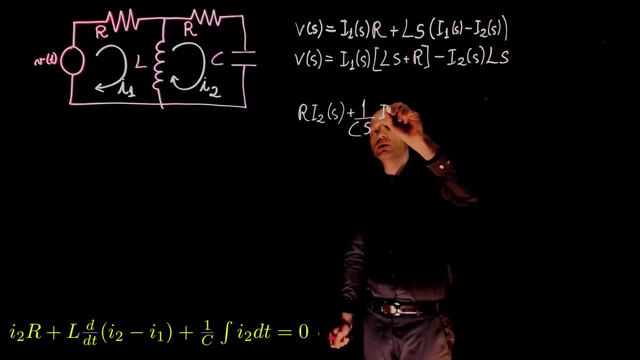 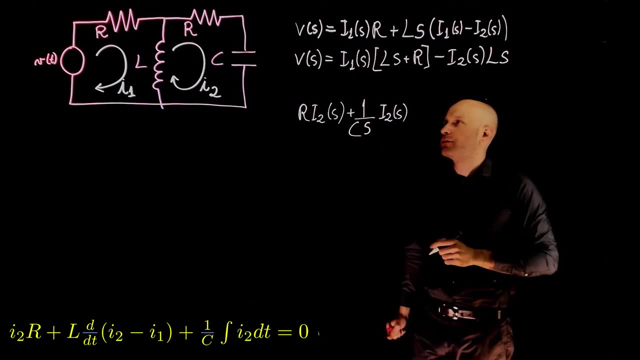 So 1 over Cs, integral of I2 of S. Again, 1 over S represents I2 of S And V of S represents the integral of I2 of S, And plus the voltage drop across the inductor again. So plus Ls, the derivative of the current I2 of S. 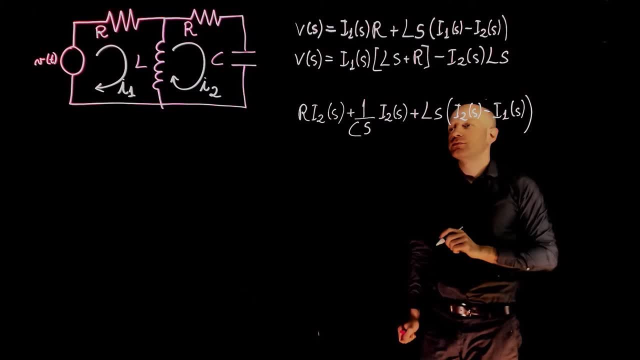 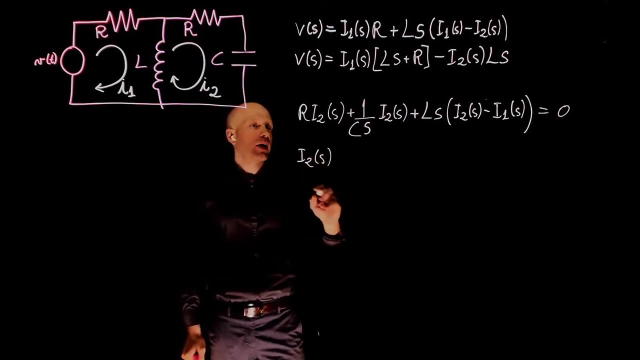 minus I1 of S, And this is equal to 0.. We can now factor I2 and move I1 to the right side of the equation. I2, that is, I1 of S, is equal to 0.. of S multiplies R. 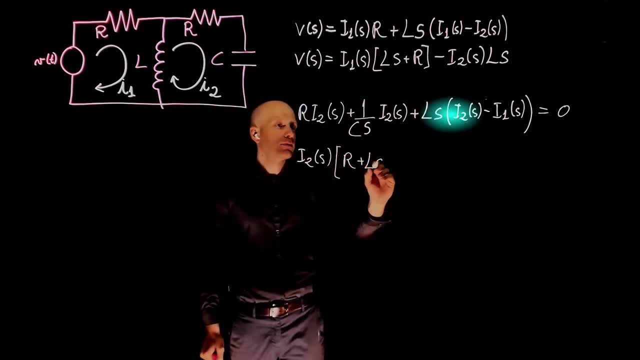 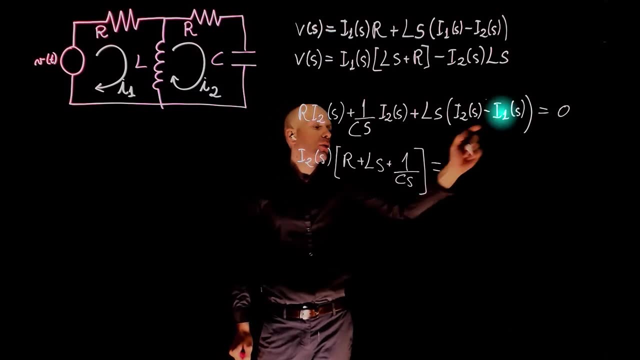 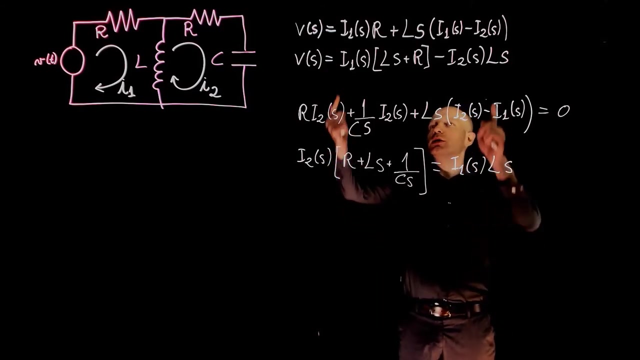 plus LS, plus 1 over CS- and this is equal to I1- becomes positive when it goes to the right times. LS. Since we are interested in the relation between I2 and V, we can isolate I1 here and replace in the first equation The expression for I1. 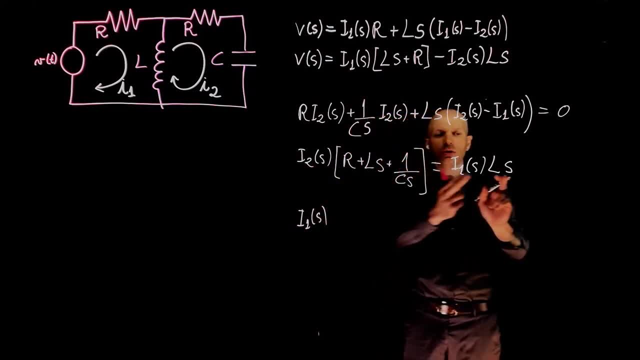 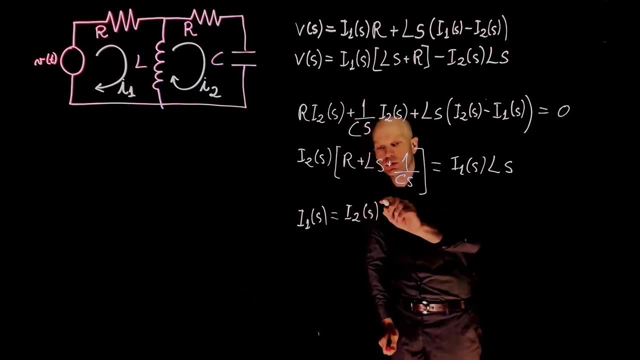 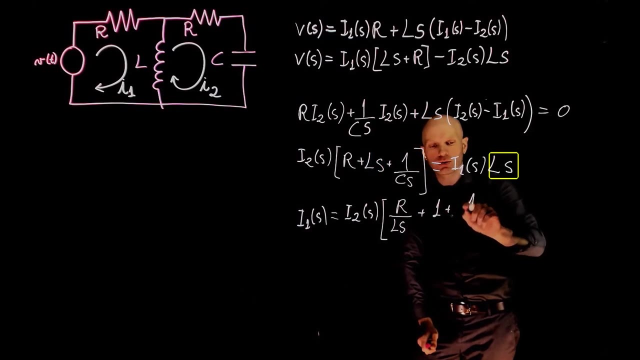 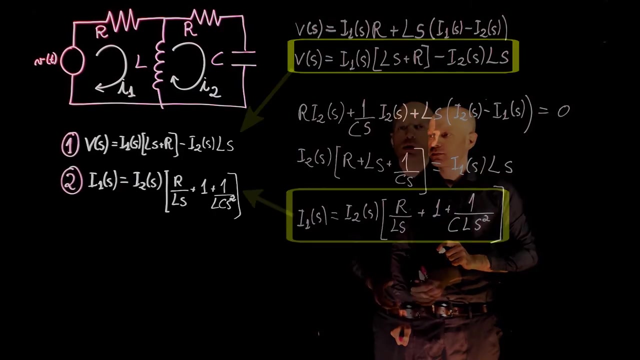 of S is this side of the equation divided by LS, that is, I2 times L divided by LS plus 1 plus 1 over CLS square. having obtained the two expressions, we can now replace I1 in the first expression and relate I2 to V. 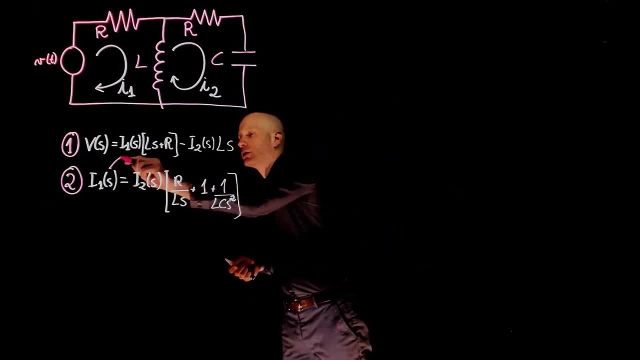 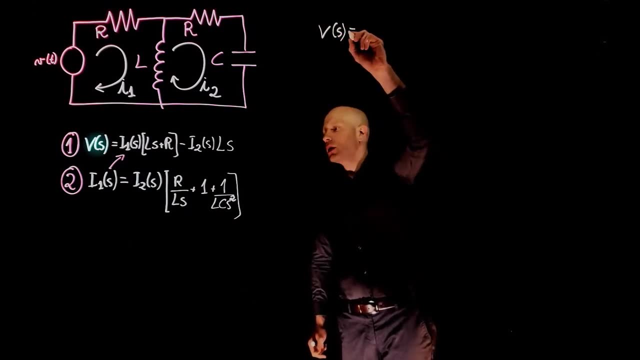 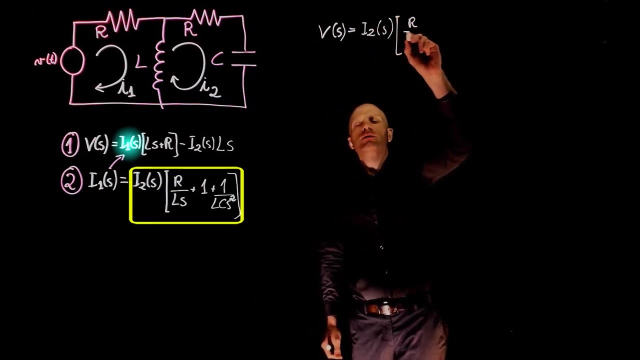 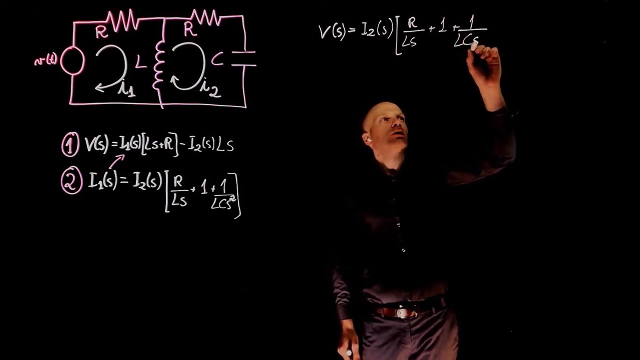 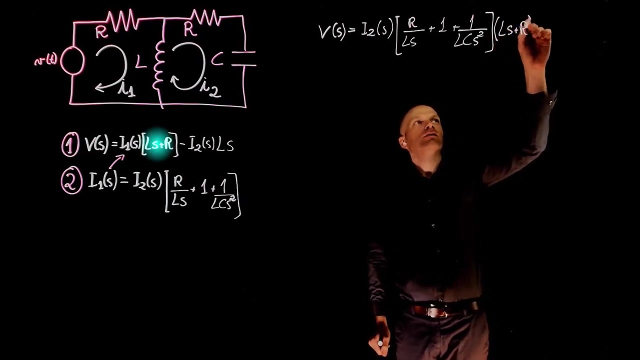 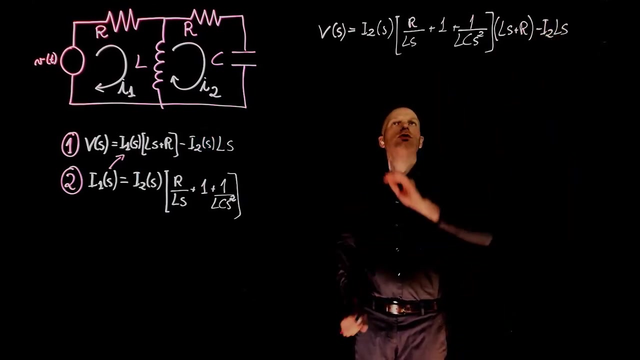 directly. So if I1 is replaced there, the first expression rewrites as: V of S equals to I2 times L over LS, times L over LS plus 1 plus 1 over LCS, squared times LS plus R minus I2 LS. Since I2 multiplies both terms of this equation, we can divide VS by I2. 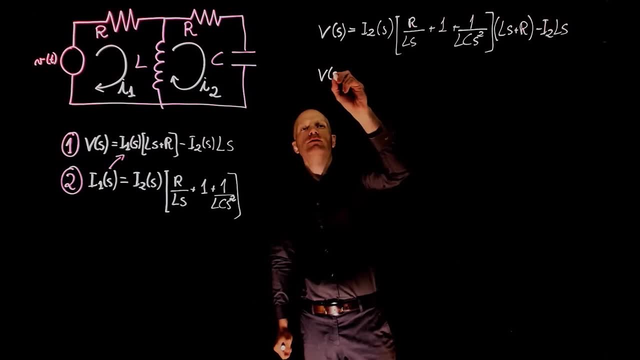 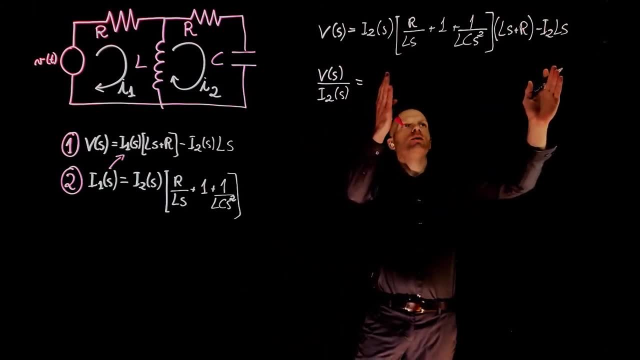 or divide both sides of the equation by I2. That gives V of S divided by I2 equals V of S divided by I2. And we then know that there isbb. we could consider V or some other HER DIFER. Then let's try FO, so we can try FO. 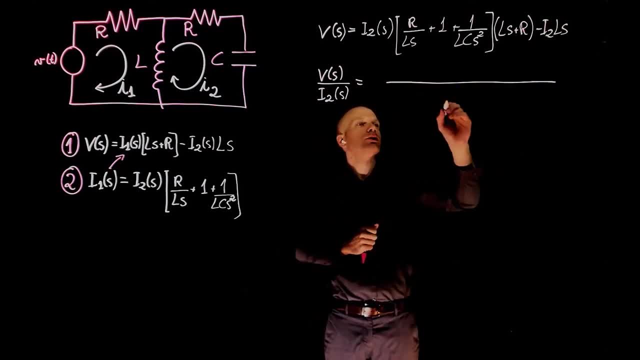 This will mean we will blink, for example. So we think that this is a movie to which we have 4 papers. The list of HU can be read like this: the dictionary, the calculator, social indicator, everything. However, these were different during this project. 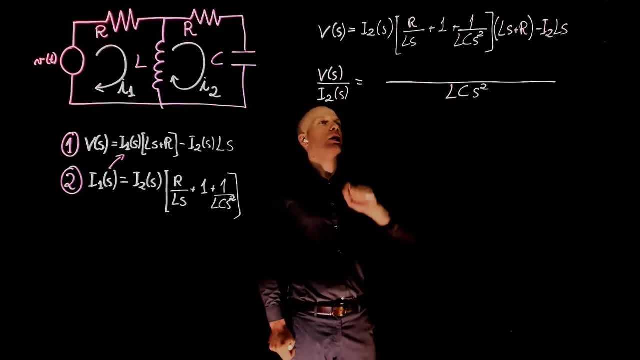 So let's work on different parameters in the fields and find out what they are and, step-by-step, we can solve them. Well, for example, we have the already Hotel and a 간단 chart, and we have several lei Santiago demonstrated whilst we were at work. 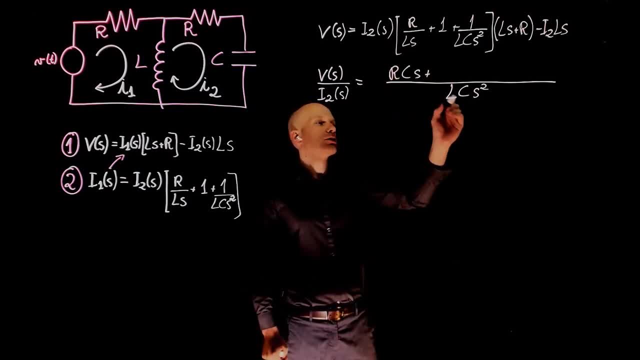 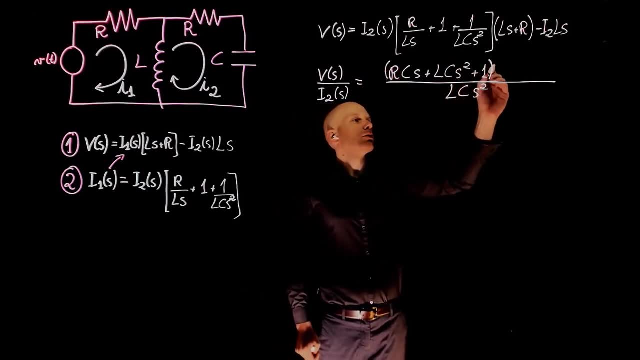 Or is it brief and we are sure to do this later. So whether we do some simple necessity analysis instead and 보여 지 σας. multiplied, of course, by Ls plus R, Lcs squared divided by 1 is Lcs squared times Ls gives L squared. 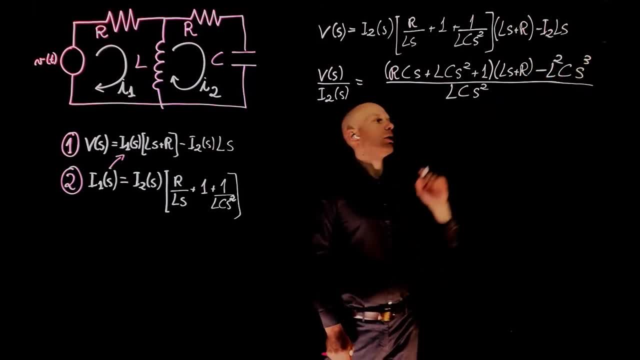 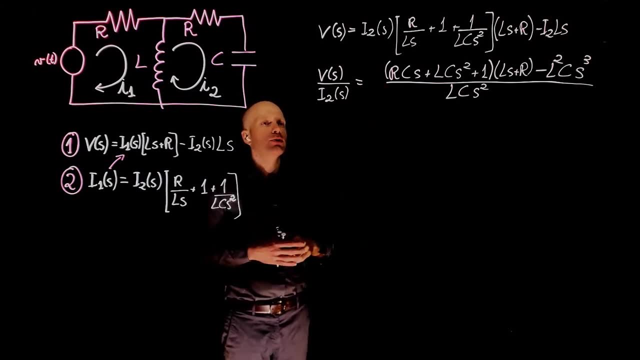 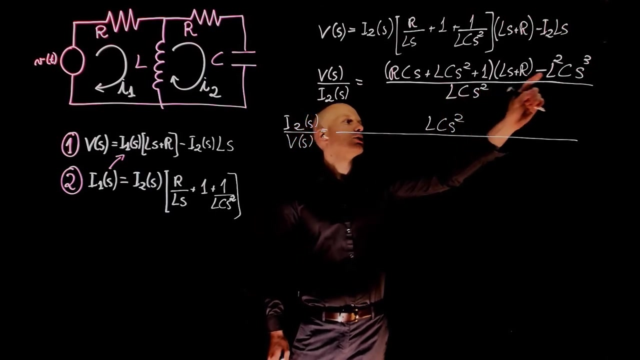 Cs to the power of 3. The transfer function is defined by the output divided by the input, which means that this expression needs to be inverted. We can rewrite it as: I2 of S over V of S equals to Lcs squared divided by the multiplication of these two terms minus the last one. 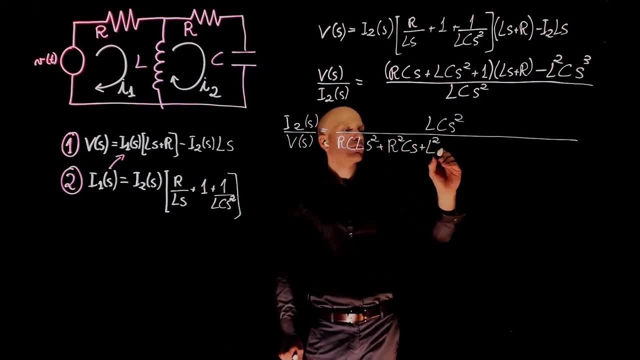 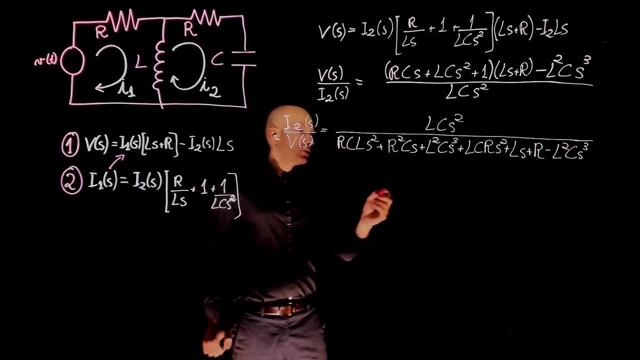 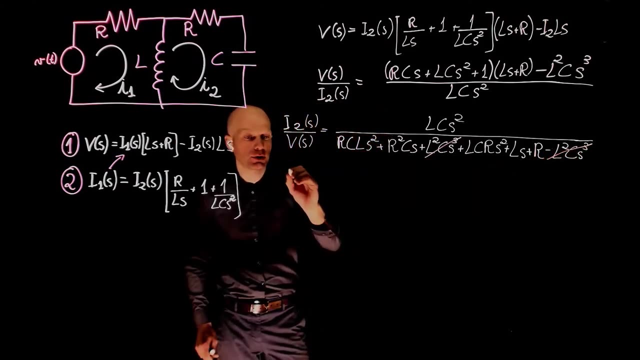 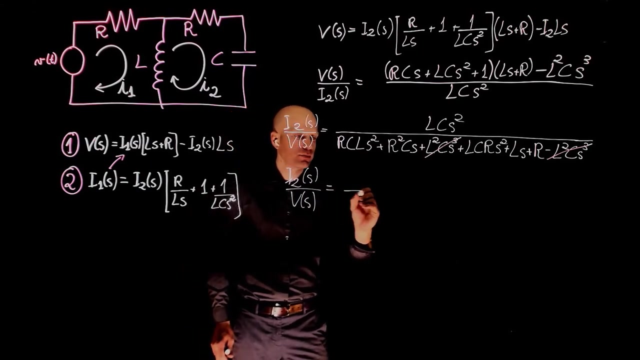 Expanding this gives this long expression. We see that these two terms to the power of 3 will cancel. So we can rewrite it as I2 of S over V of S And you can further simplify this expression: I2 of S over V of S equals to Lcs squared. 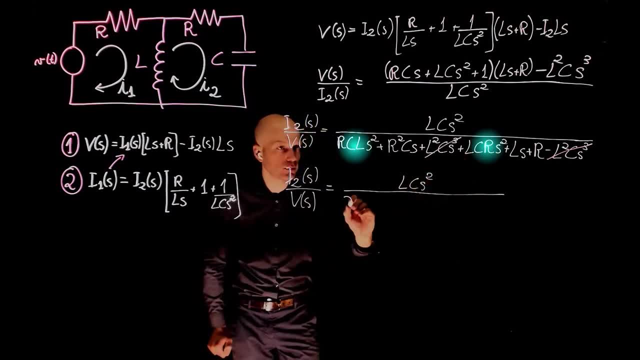 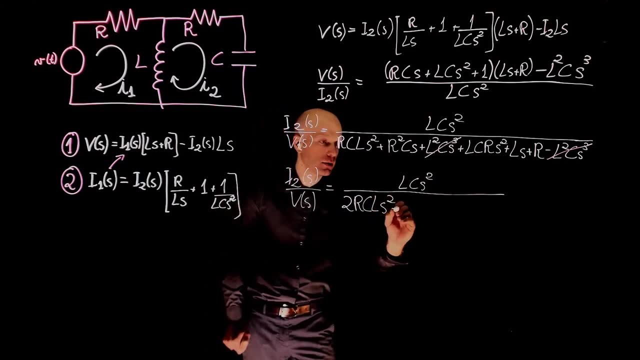 Starting with the power of two terms. We have 2 Rcls squared And now we can factor all terms with S plus R squared, C plus L, and we have 2 Rcls squared times S plus R. And this is now the transfer function between the output I2 and the input V of S. 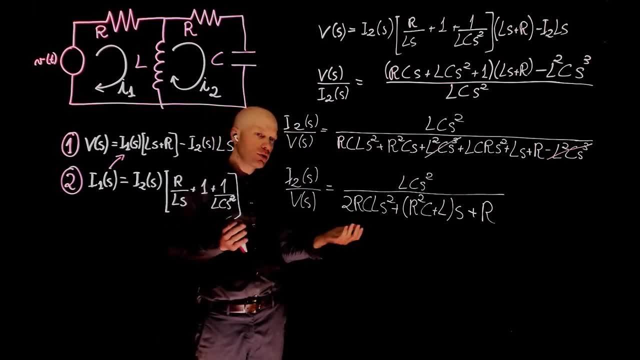 Now let's go one step ahead and assume, for instance, that instead of I2 we were interested in the voltage across the capacitor as the output of the system. Let's say Vc. Here we have I2 of S over V of S. This expression gives I2, provided that a V of S is applied to the system. 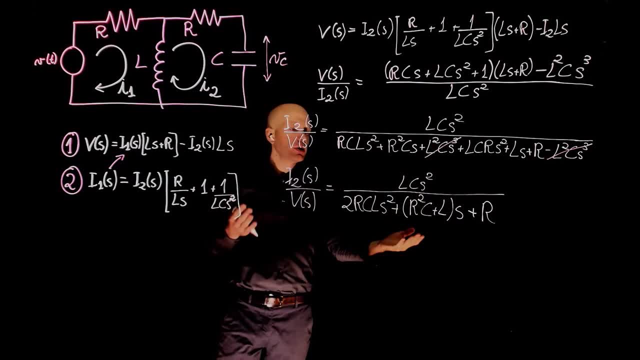 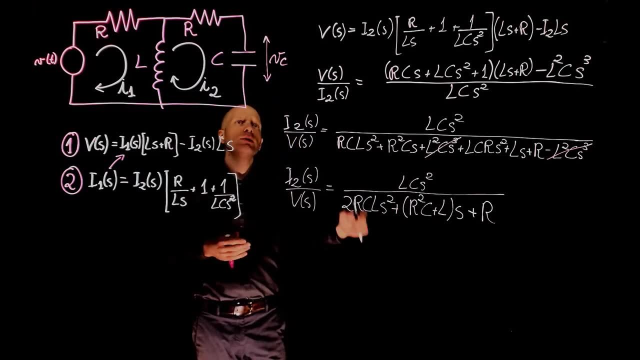 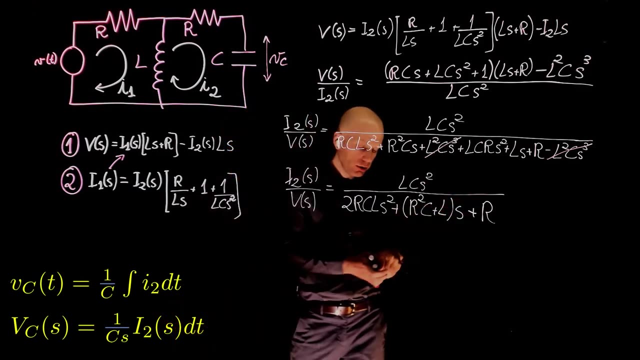 If you want to go from this to Vc, What would be the procedure here? Thinking about this as the current, To go from the current to the voltage, We would need to integrate the current and divide that by C, Which means that if we multiply this expression here, 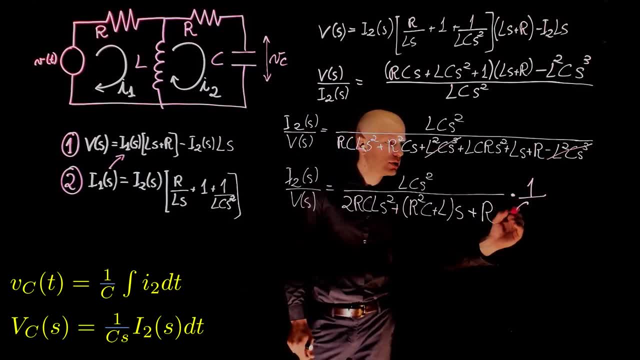 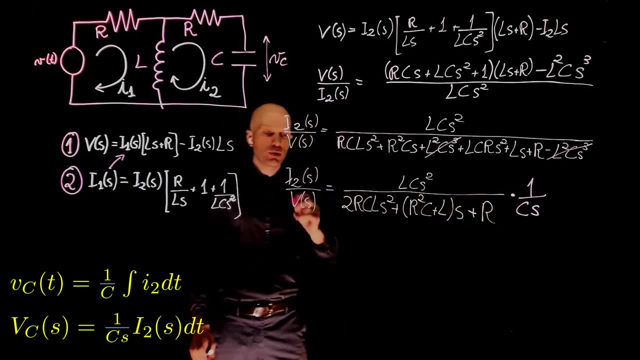 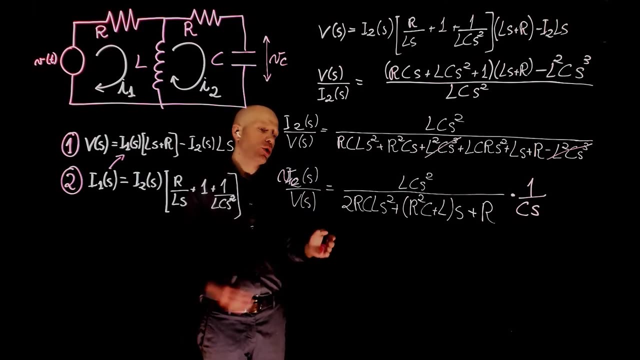 by 1 over Cs. We are taking the integral of this expression and dividing that by C, Which means that now I2 becomes Vc And it would go from the current to the capacitor voltage.